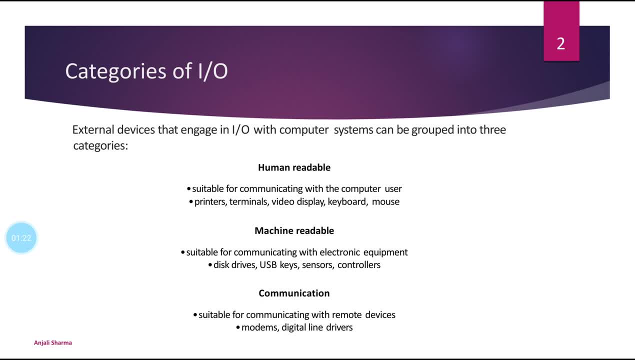 readable. Next we have machine readable. It is understood by the name: those input output devices whose basic functioning or the data that is being displayed on the screen. So the data values we have are understood by the machine, meaning those that work in. 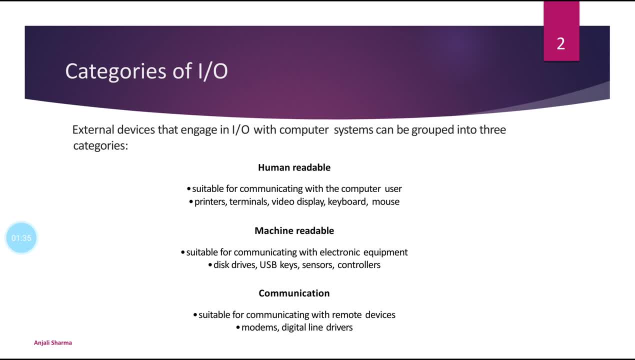 the format of amplitude or those that work in the format of binary. So what is happening with USB or your disk drives? suppose that you have sensors that works in data collection. they are coming under this, Basically those who deal with binary data. The third category. 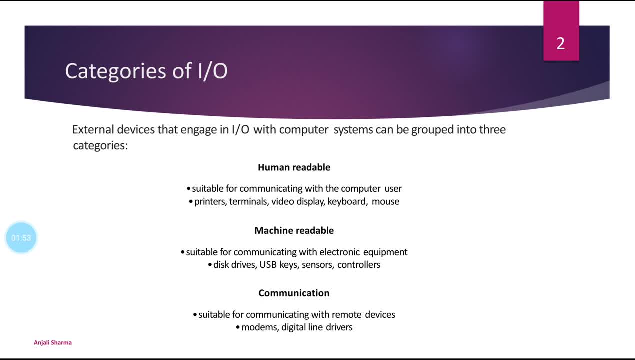 that comes here is communication, and here communication means those devices which are used for translation, transferring a data from one system to another, that is, those devices which are used for communication. they are IOs of your communication, For example modem. Everyone knows that in internet connection. 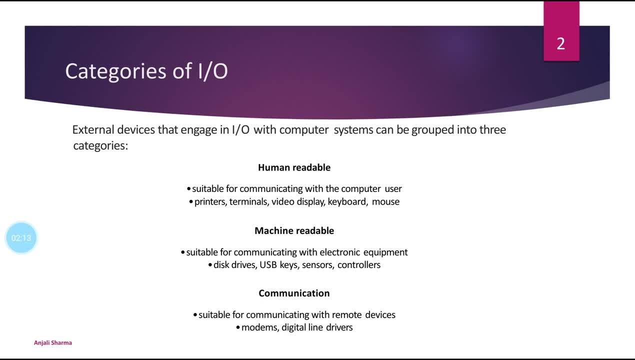 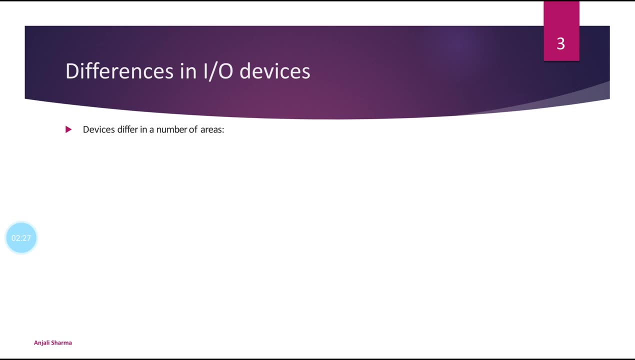 we have the requirement of a modem which connects us to a remote system and basically, in networking, we have it in usage. So these are different types of IO devices. Next, what we need to know is the basic parameters on which these devices. now, we have seen only three types of devices, but there may be certain. 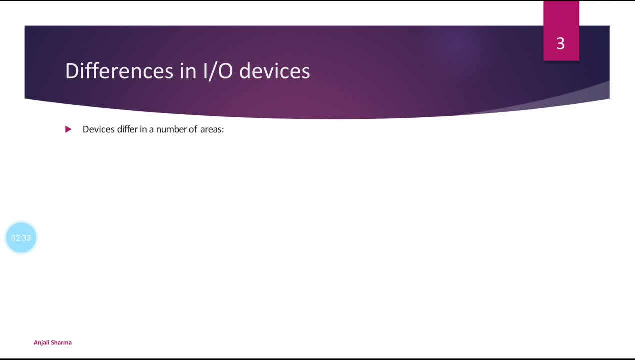 parameters on which we can differentiate them, that how one input device differs from the other input device or how it can be better, or, basically, if we have to make a choice that in a particular scenario which IO device should we use, then we should know these parameters. The first parameter we have is data rate. 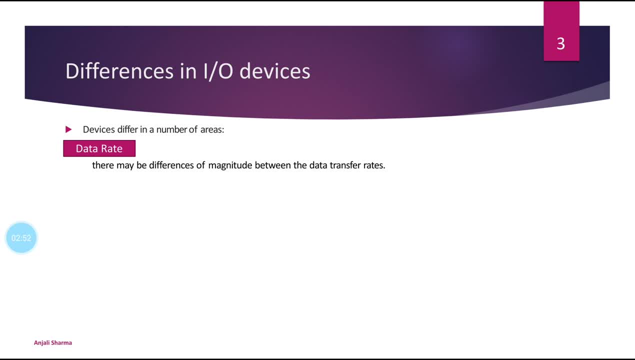 Data rate means how much time is taking for data transfer. Suppose I have an input device, I have a keyboard, I pressed it, then how much time did I get data? how much time did I keep it in memory? that is the data transfer rate. that is the data in and out time. 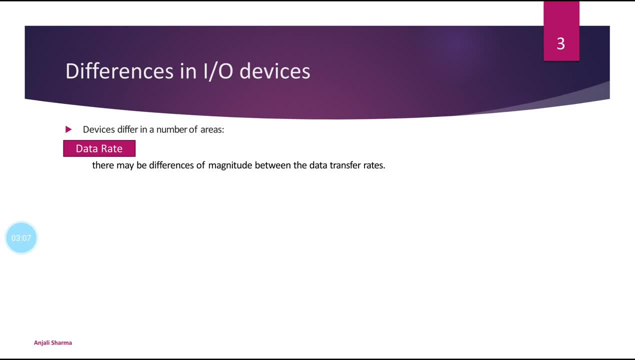 So there may be differences of magnitude between the data transfer rate. Next category which comes is application. Application is the use that. for what use are we using that input output device? according to that, our software will be made. That means that if I am activating any input output device, 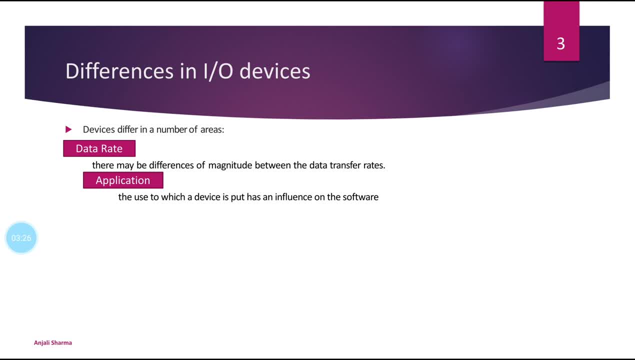 means. how do I want the output? I want it on the screen, or I have to print the output, or I have to keep the output scanned. if I have to enter the data, then it will be on the signals, that is, on the commands, which can be done through your mouse. it can be done through the joystick. 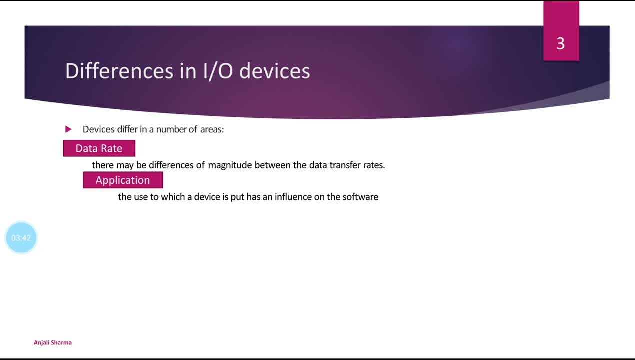 or the keyboard, which works on signal conversion. So, basically, what is the application? Next comes we have complexity of control. See the meaning of complexity of control here. we know that there is a kernel in the operating system where all the functions of the operating system are stored. 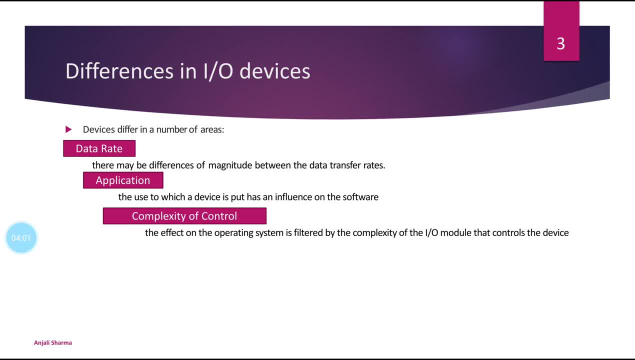 So one function will be the input output management of the kernel. Now in input output management we are managing I-O devices. corresponding to each device there will be a device driver, that is, there will be a software program which will be controlling that device, means its controller. 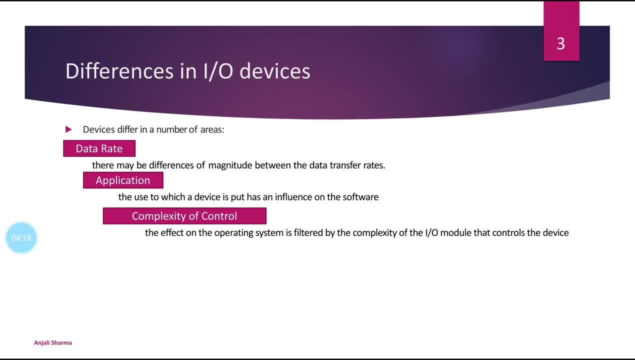 So what will be its complexity? We should also know this. it depends on whether your I-O device is of what kind, and basically on the basis of that the complexity of your operating system also depends. So one complexity of control should be known. Next, that is unit of transfer. 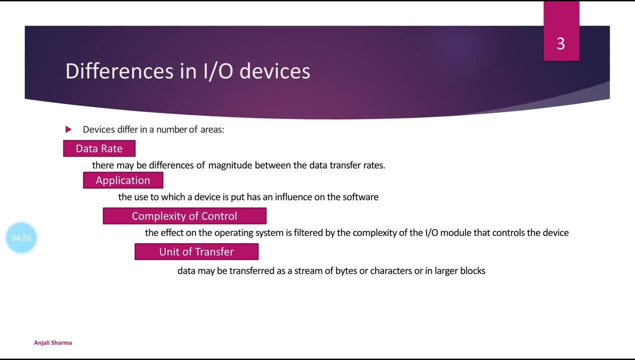 Unit of transfer. now we have also seen in the data rate that the data is going in and out, because in input output devices the data goes through the input and if it is read from the memory it also comes out of the memory through the output devices. So that is the unit of transfer. 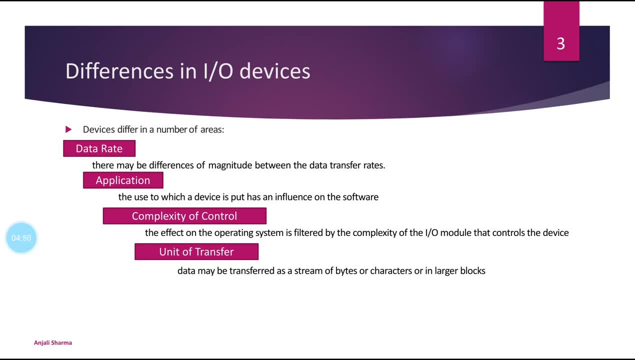 data is coming in bits, it is coming in bytes, it comes in blocks or it comes in streams. it is being transferred. So that is the transfer unit. Next, we have data representation, Meaning in which format are the input output devices representing the data? 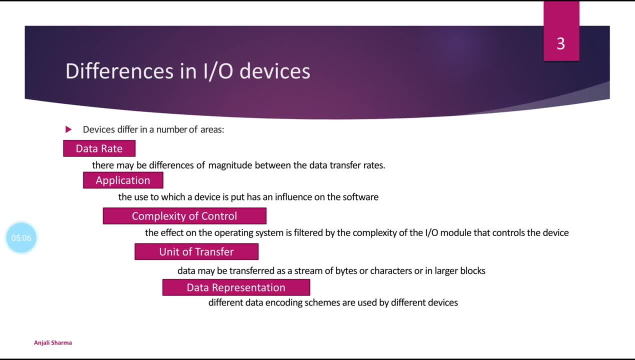 Either they are working on SKI values or they are working on Unicode values. Is the representation of 32-bit or 64-bit? I mean, this is the basic representation of data, And the last one is the error condition. Now, what is the error condition? 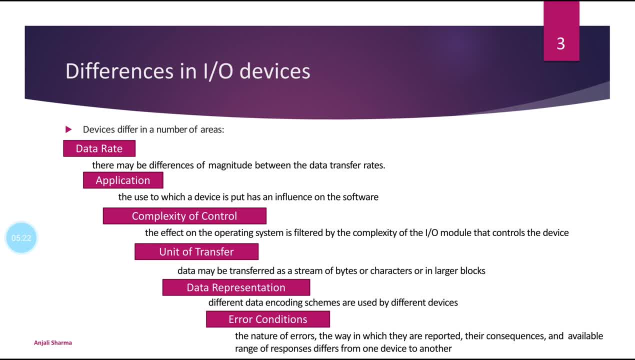 Whether we work on any software or hardware, basically the IO will be a combination of hardware and software, because the device will be hardware and the module written to control it will be a software. So if we talk about it, then errors can come in both of them at any time. 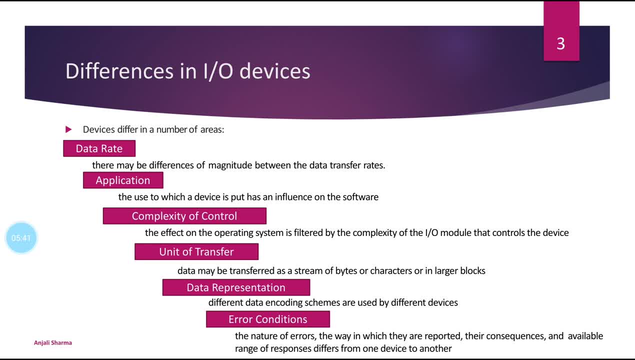 Errors can come in software, bugs can come and there can be a fault in your hardware. So if there is a fault, then how does your IO device manage it Right And, to represent it, what is its response? If there is an error, then how the IO device is responding. 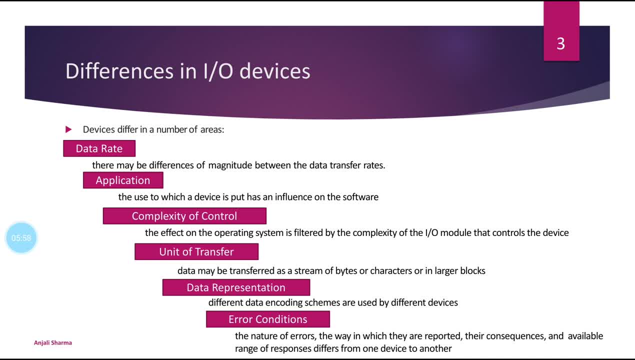 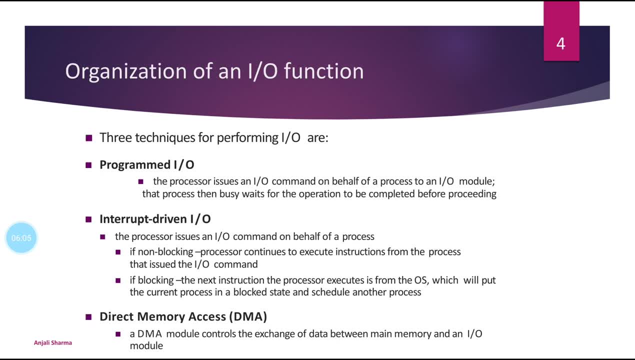 So on the basis of that, we can differentiate. So these were certain areas through which we can differentiate the input output devices. The next topic is that you need to understand the basic working of your IO function. First of all, let's understand what is IO function. 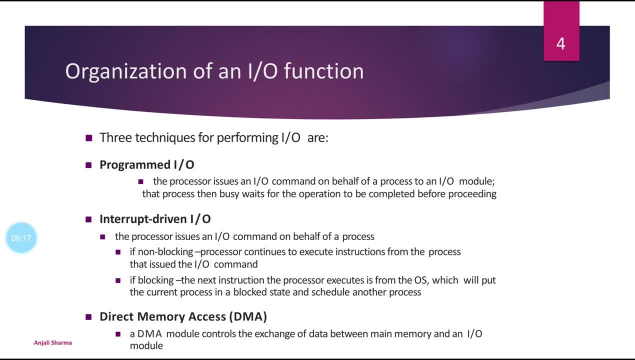 IO function is the working of input output. Basically we need input output. So an IO request is generated, The operating system handles it And it sends the command to your CPU. CPU basically performs Means that IO generates the request and processes it. 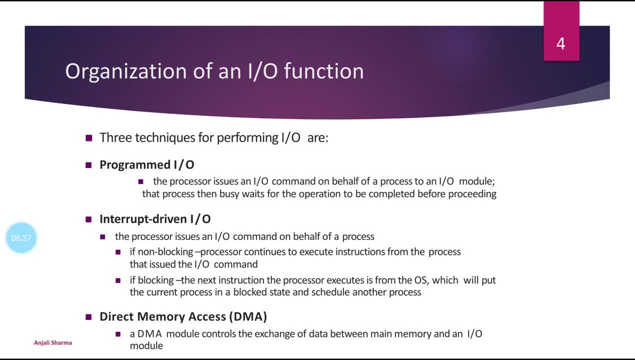 Right. So this whole functioning meaning I need a data. So I generated an IO and gave input. I had to store that data in memory. So in the input device your keyboard is activated, The data goes through the keyboard. 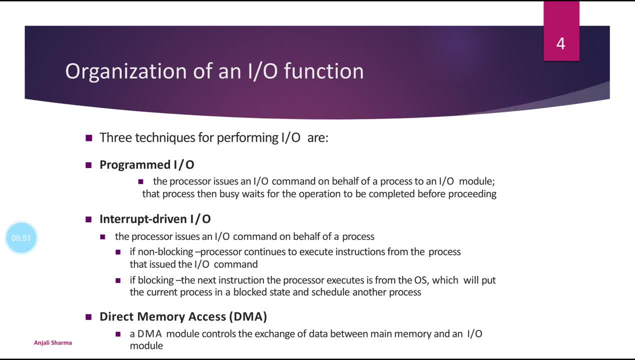 The data is converted And stored in memory. To store in memory and for conversion a command is run, That processor runs it. So basically in IO function your CPU memory and basically IO devices and drivers are involved. 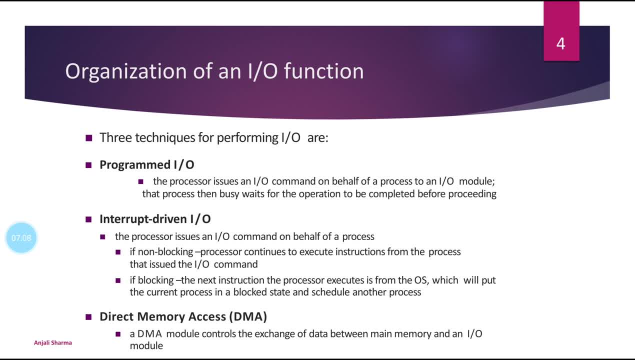 So we have three ways to do this IO function: First, Programmed IO, Second, Interrupt Driven IO, And the third is your DMA, That is, Direct Memory Access. You must have read all these things in your computer organization. 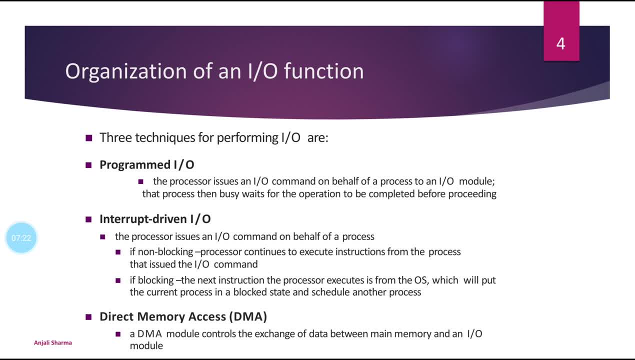 Here you should know only its general introduction. Like Programmed IO. So if we want to perform IO function, we will perform it programmatically. It will be written in our process code And what our CPU will do. 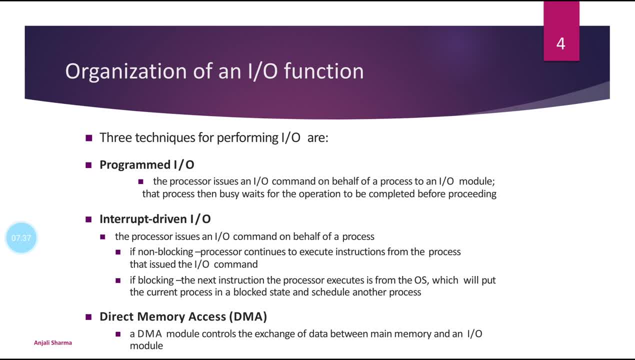 It performs all the things we have written for IO in its code. What is in Interrupt Driven? Your programming efforts have been made a little easy. And what does your code do? It generates an interrupt, Operating system handles it And processor acts accordingly. 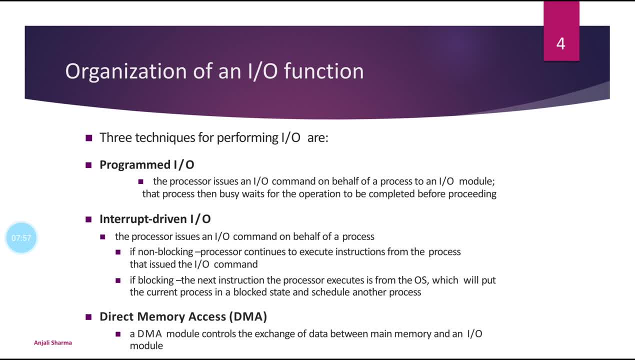 So what did we do? We removed our programming and put it on Operating System, So the handling mechanism went towards Operating System. Now we have two ways to do this. Either our CPU will be blocked or it will be unblocked. 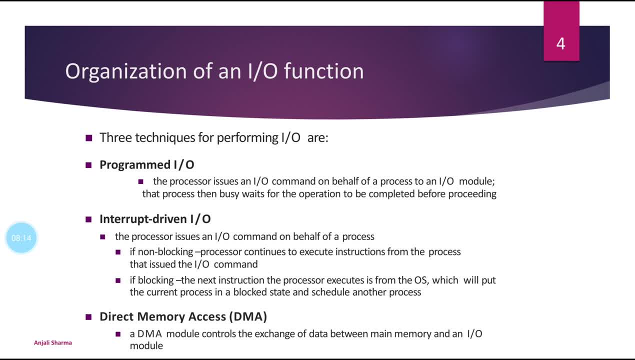 If it is blocked, then at the point of time IO is functioning, the processor cannot perform any other task. That means it will remain idle or in busy waiting. It will keep checking whether IO function is completed. If it is completed, then it is okay. 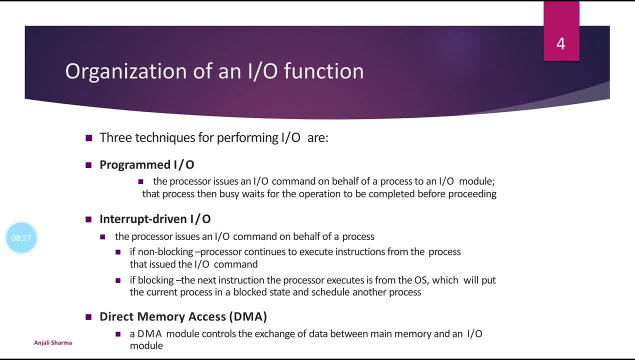 Otherwise it will wait In non-blocking. it can perform any other task at that point of time, Which is obviously the better option. The last one we have is Direct Memory Access. Direct Memory Access is a very important topic And to write a short note on it, 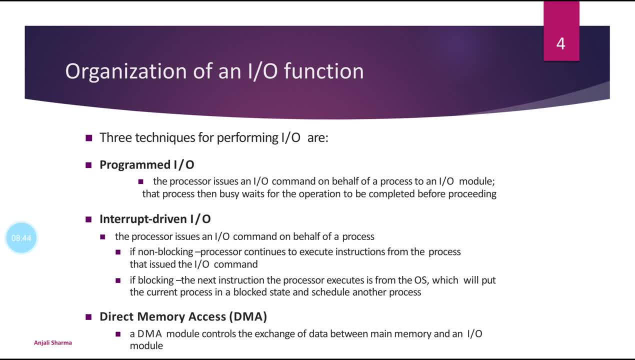 Karib University has asked twice in the last five years. So let's talk about DMA. You have also read this in detail in Computer Organization. Here you should know its basics. Peripheral devices directly access the memory. So the DMA controller concept that you have. 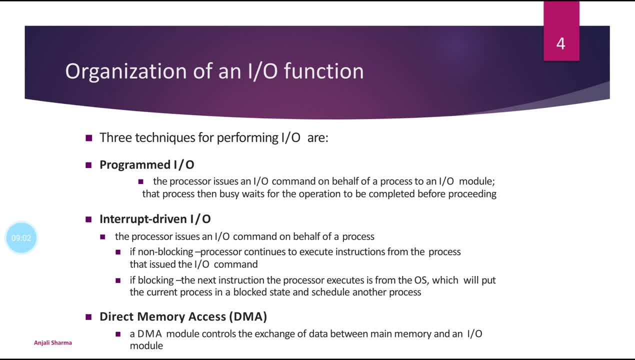 what does it do? It can directly access the memory through your data buses, address buses and control lines, So you don't need to access the memory through CPU. So that is a better option. So you have to read this in detail. 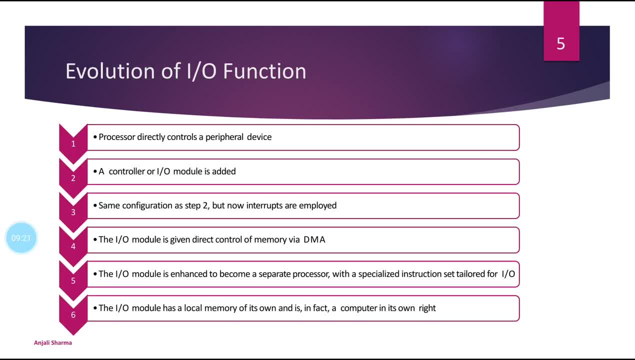 The next thing that we should know is the evaluation or evolution of these IO functions. IO functions means the input and output, the operations that we have, how they used to happen and how they happen now. So what changes came in this with time? 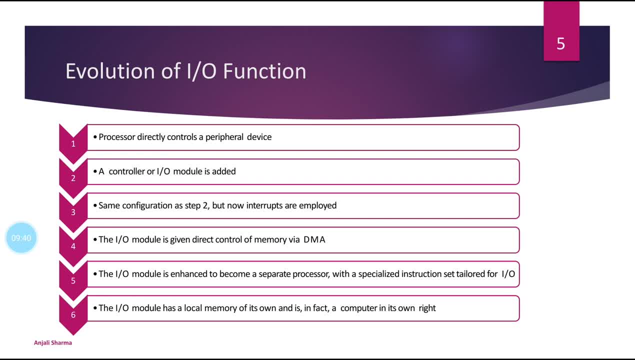 So, first of all, the processor that directly controls the peripheral devices. Before that, your CPU used to do all the tasks. After that, what we did? we attached a controller, That is, a software that controls the input and output devices. 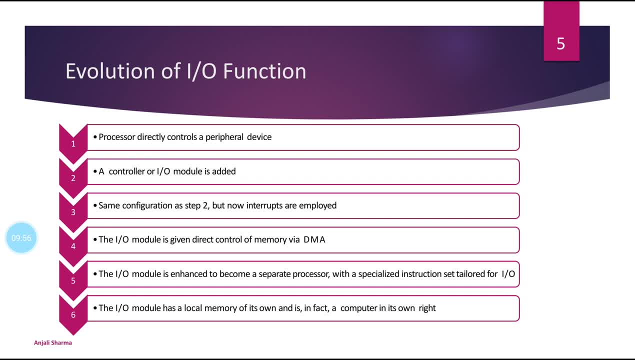 We introduced that. After that, in the second step, we made it interrupt driven. That means we gave the task to operating systems That most of the IO functions will perform OS. After that the introduction of DMA came in. 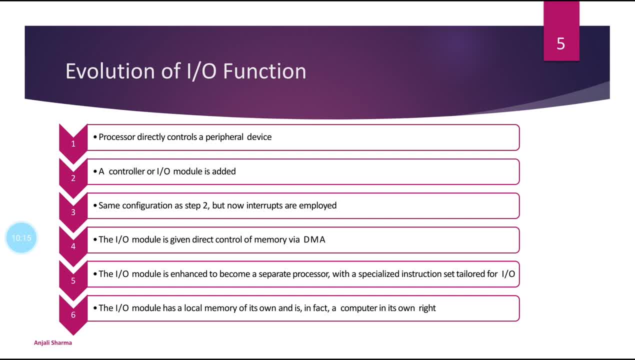 That means we directly started accessing the memory of peripheral devices. Fifth, if we see what changes came then we added an IO module. You can understand the IO module, that now two processors are given in your system. One processor will process your processes. 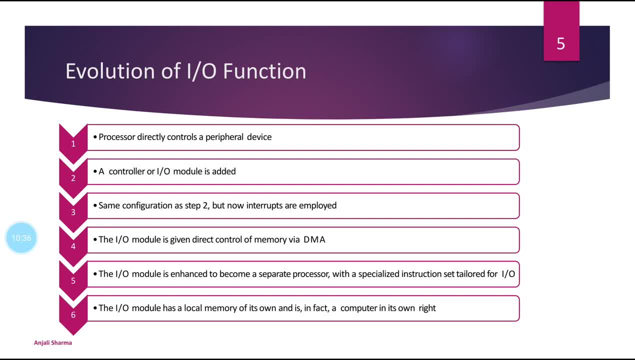 means it will execute them And one processor will do the dedicated task for your input and output devices. So it will never have a processor, It will never have a processing, It will never have a calculation task. All the IO requests will go to the processor of your IO module. 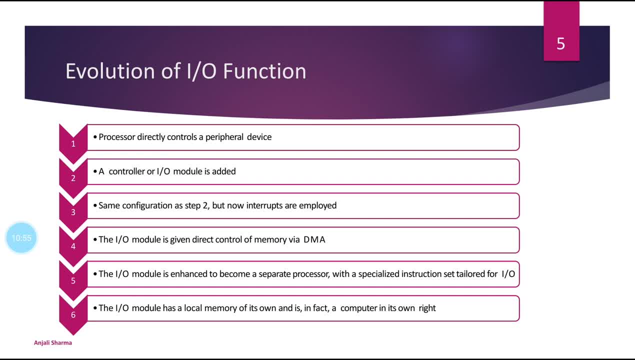 So two processors: One which is dedicated to input-output operation And other which is for the normal processing. The last concept that we have now is the one with two processors, But your IO processor. there are two processors in the main system at this time. 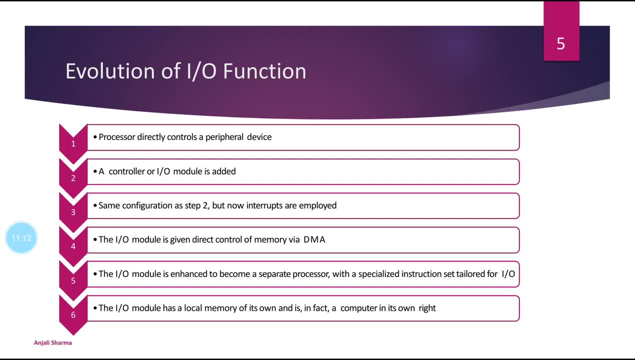 So the IO processor. it has a small memory, So now it is like a small computer in itself which basically performs the input-output. So now in your system you understand that there is a portion in which there is a dedicated processor. 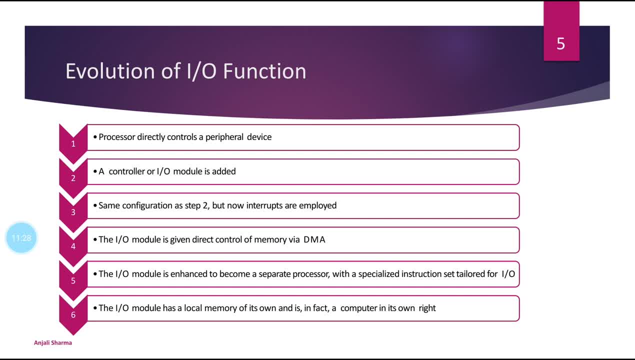 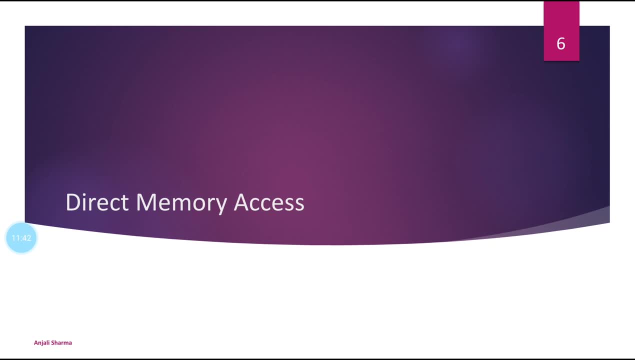 It has its local memory. So whatever task will be related to input-output, your IO processor can complete it. So in IO functioning by the time so many changes have come, A little discussion on DMA, because this question is asked in your university. 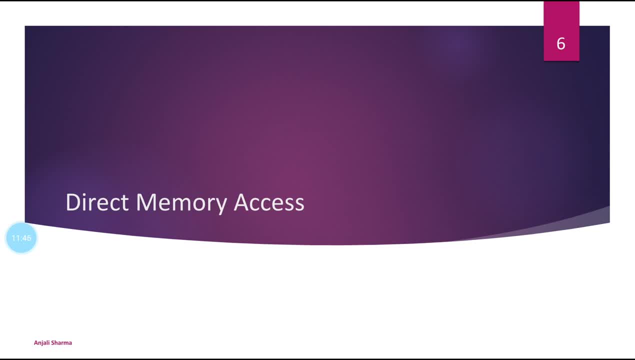 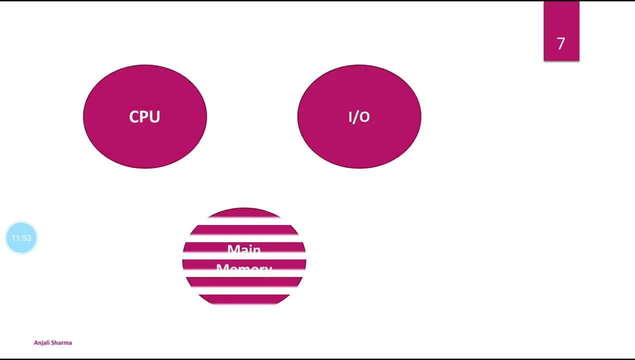 So, basically, what is direct memory access? Let's understand it in a very simple way. Suppose you have a CPU and you have input-output and you have main memory. So you have these three modules. Suppose we have to access the main memory. 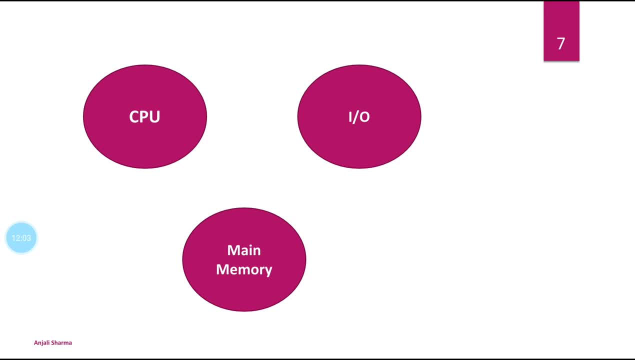 and have to access through input-output. Suppose we have to keep any data in memory or have to read from memory via input-output devices. So what used to happen earlier? that input-output devices used to contact the CPU for this and the CPU used to contact your main memory. 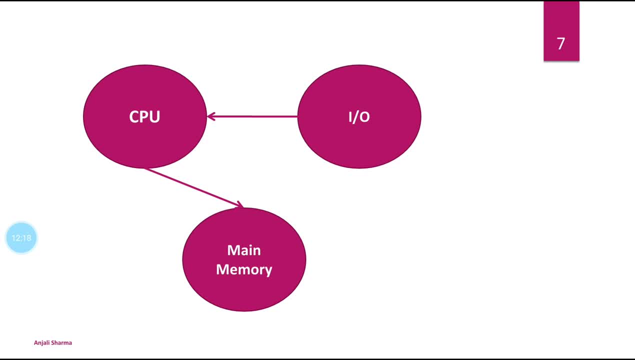 Because when we studied the fourth unit, even then it was taught that the CPU has direct access to the main memory and no one else has it. So IO devices had to go to the CPU's through memory. So that means 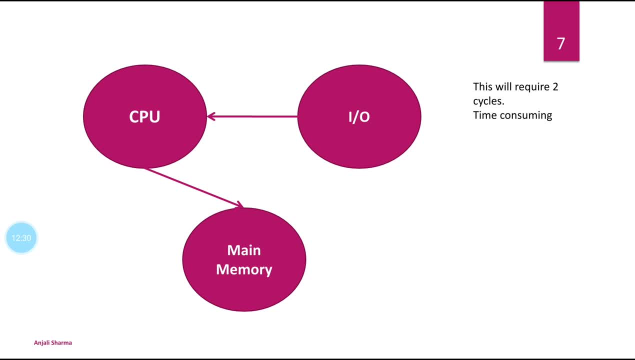 we have two cycles here and that is time-consuming. So what was done now? We directly thought that can it not happen that IO devices can directly access the memory? So obviously, instead of two, it will take one cycle. 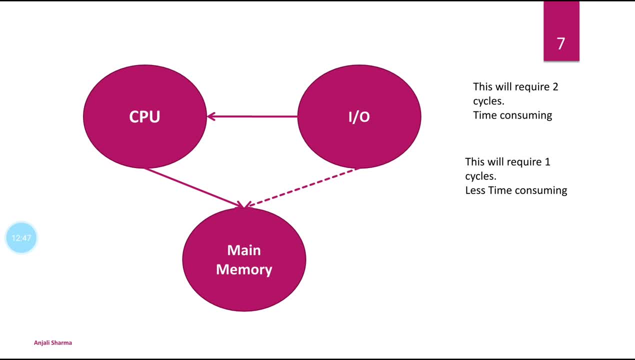 and that will be less time-consuming. So in this scenario in which input-output devices directly control the main memory or can access it, for that we made a DMA controller which we read in DMA Direct Memory Access. So now IO. 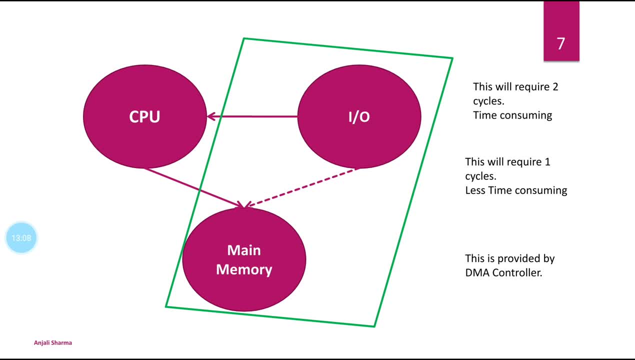 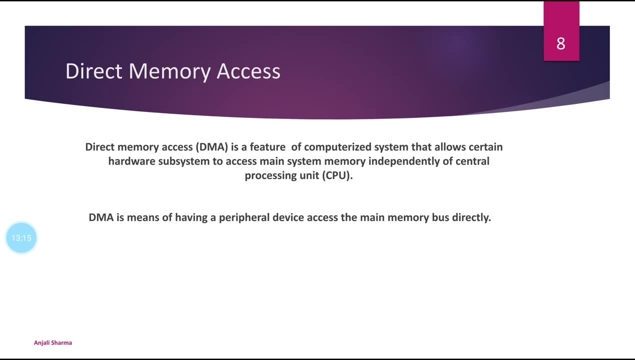 ie, peripheral devices, which we generally call, can directly access the main memory. That is the concept of Direct Memory Access. If we talk about it, Direct Memory Access is a feature of computerized system that allows certain hardware subsystems to access main system's memory independently of your CPU. 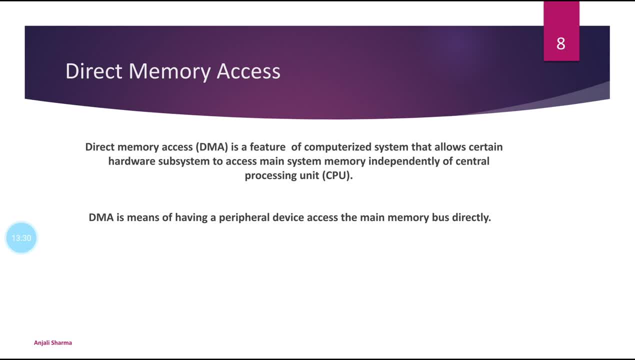 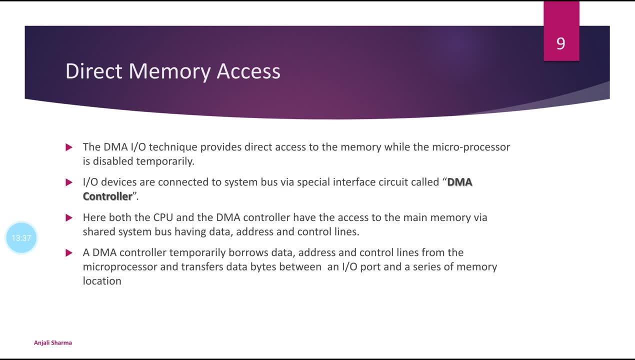 So instead of CPU, it directly accesses it And it means of having a peripheral device access to the main memory bus directly. So basically what happens in DMA: the technique of DMA is to directly access the memory and we do this through DMA controller. 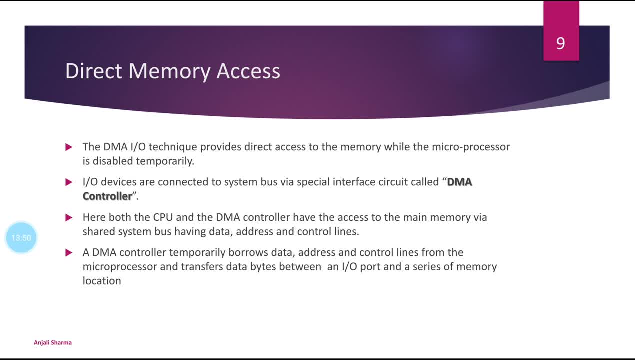 Here both the CPU and the DMA controller have the access to the main memory via shared system bus having data address and control lines. A DMA controller temporarily borrows the data address and control line from the microprocessor and transfer data bytes between an IO port and the series of memory location. 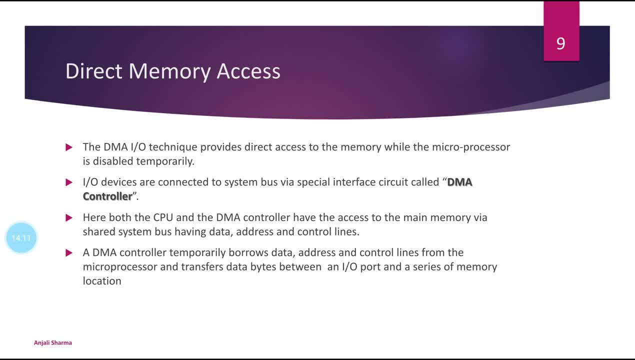 So by bypassing the CPU, we can directly access the memory. This improves our transfer rate and it is also less time-consuming. Plus, we also free the CPU for more tasks because it is now completely free from handling IO requests. 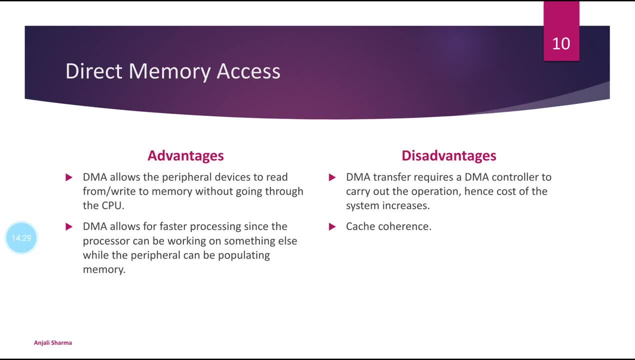 Some advantages and disadvantages of DMA. Again, DMA allows the peripheral devices to read from and write to the memory without going through the CPU. Plus, it allows faster processing, since the processor can be working on something else while the peripheral devices are accessing or populating the memory. 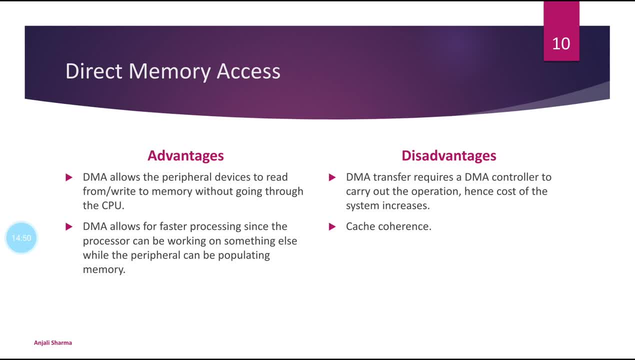 Talking about the disadvantages. DMA transfer requires a DMA controller to carry out its operation. So definitely, we have to write a DMA controller and there is a slight change in the hardware, So it is a little bit expensive. Plus, we have a cache code.